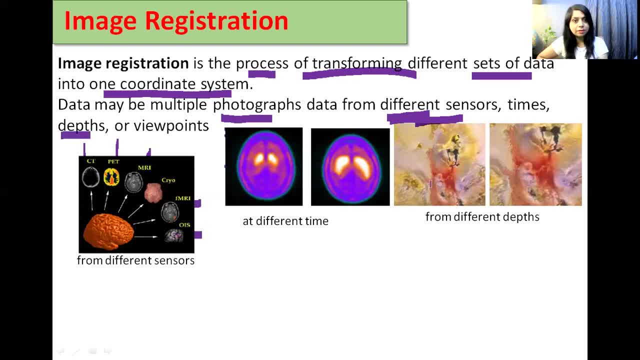 or images are taken from different depths. different depth means, uh, images are of different sizes. you can say: you can see, here this is taken at different depth and this is very closer. these are jupiter images. so here, this is very close view and this is a far view of the same object, that is jupiter. so images. 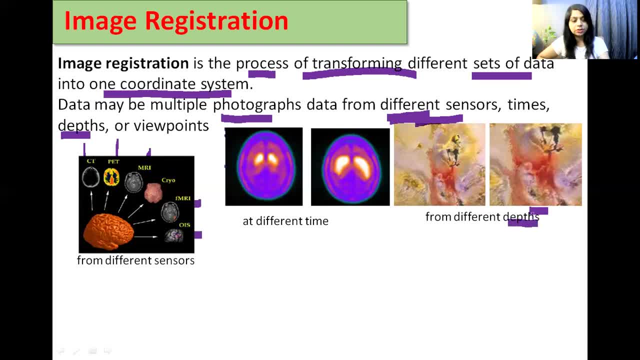 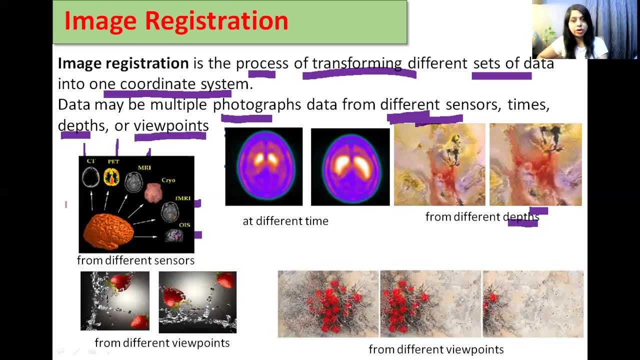 are captured with different depths or the images are captured from different viewpoints. what is meaning of different viewpoints? you can see here the object is same, this is a very image, but here the camera is rotated. or here also you can say: this is images, image of one scene, here flowers. 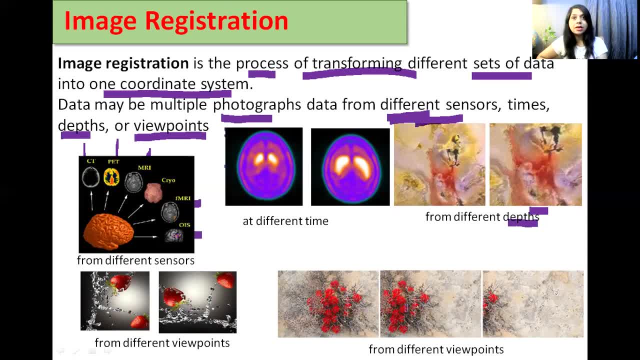 are exactly the same, exactly at the center of the image, and then a camera is spanned towards right direction and now the flowers are not at the center. and here again, again it is: camera is spanned towards right and flowers are not at all available in the image. so you can say that these images 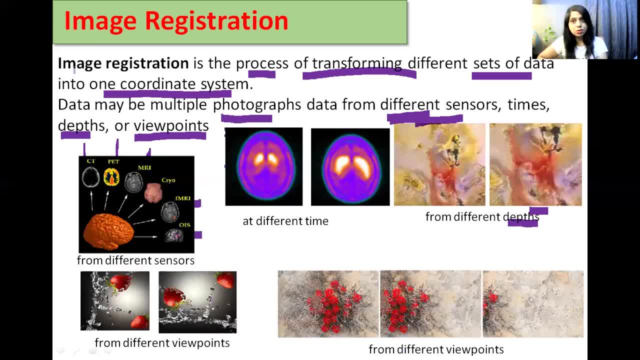 are taken from different viewpoints. that means what is image registration? now, if the images are like this- that means, if they are captured from different sensors, or if images are captured at different times, or if images are captured from different depths or from different viewpoints, then bringing them in the same coordinate system is known as image registration. again, 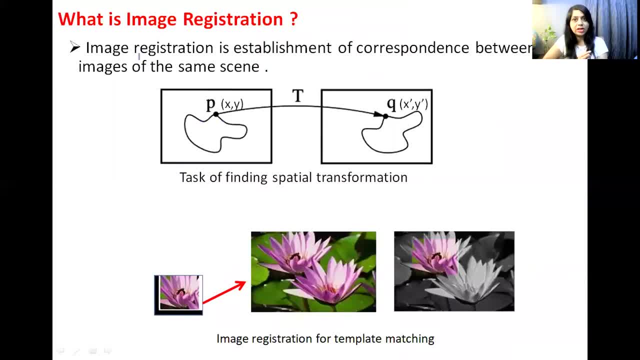 i will give you another example. what is image registration? image registration is establishment of correspondence between the two images of the same scene. what it means you can see here, this is one image and this is second image. here object is same. you can see, this is object. here any pixel p. and suppose this pixel p has coordinates. 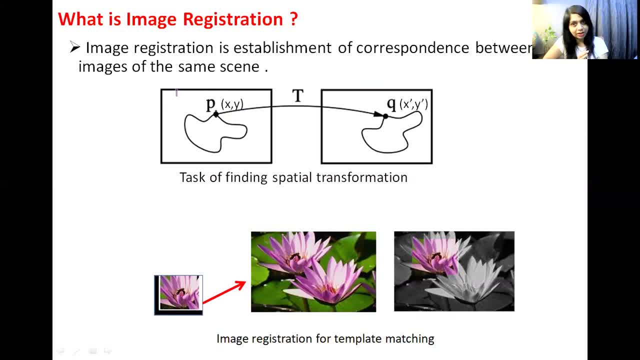 x comma y. that means x in this direction and y in this direction. this is y direction and this is x direction. now in this image, if you see, it is same scene. same scene means object is same but it is displaced from the same scene. so this is the same scene, but it is. 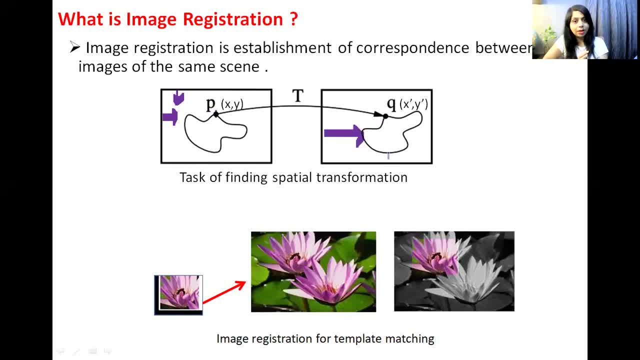 rotated towards x direction like this, and maybe a little in the y direction. it is slightly rotated, you can see here. this portion is not here, but it is here in this image. so image or object is slightly rotated and here the p point is exactly similar to this q point. 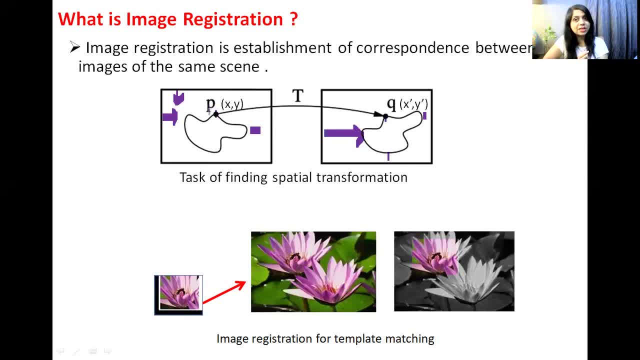 that means in the previous image: if the pixel p has coordinates x, comma y, then in this image the same pixel is same as x. in this image- and here you can see that the p point is same- gets coordinates x, dash, comma y, dash. so pixel p and q is same, but here the coordinates are. 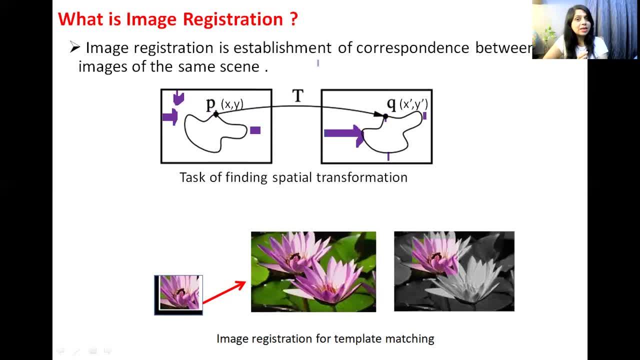 different. so image registration is establishment of correspondence of pixels between the two images. that means we have to find out what is the correspondence between p and q. so it is a task of finding spatial transformation. this process is known as it is: a spatial transformation, so aligning. 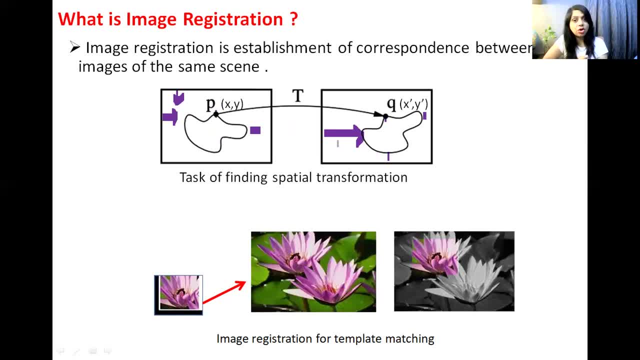 these two images is image registration. the process of aligning these two images or changing this image like this image is known as image registration. now, here you can see second application, another application of image registration you can see here. this is image and this is a template of 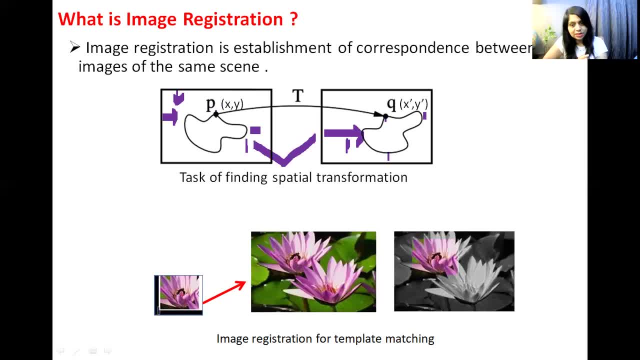 same image. so what happens here? you can see this corner, where this commerce, this, this corner. you can see this corner or this particular pixels at the corner, where it exists in this main image. it exists exactly somewhere here. that means it is same case here. so we have to identify what are the coordinates of these pixels. and then we have 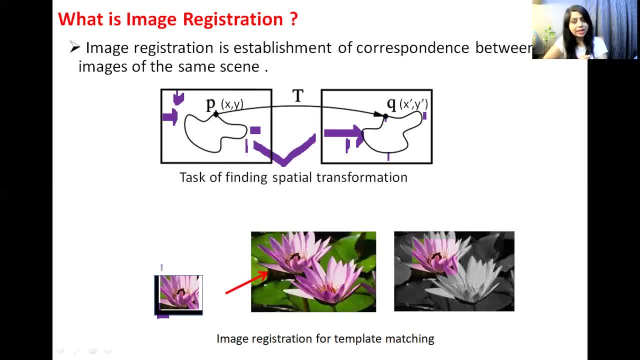 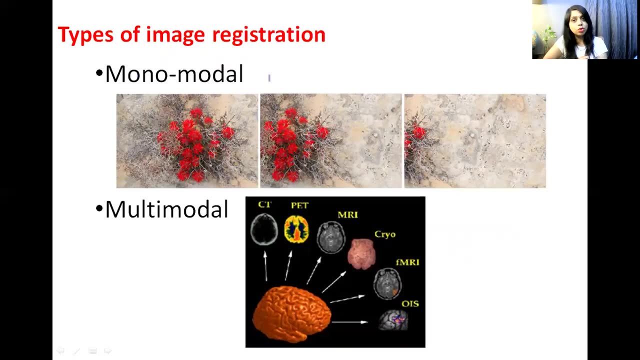 to find out what are the coordinate of same pixel in this image, and then we can align, or you can match this template with this main image. so this is known as image registration. now what are the types of image registration? image registrations are of two types: one is mono model and another is multi-model. what is meaning? 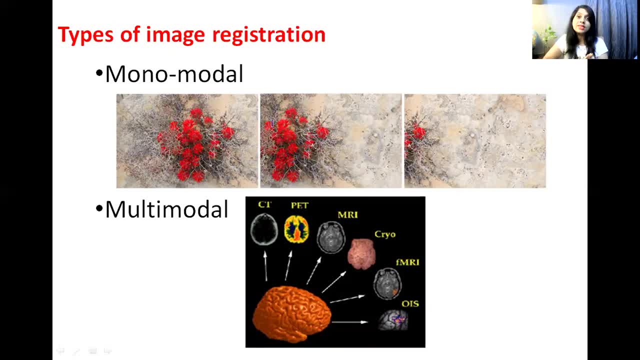 of mono model when images are captured by the same sensors- here you can see that the images are captured by same type of camera or same sensor- is known as mono model image registration. that means when we establish a quality correspondence between these kind of images. it is said that it is mono model image registration and this is multi-modal image. 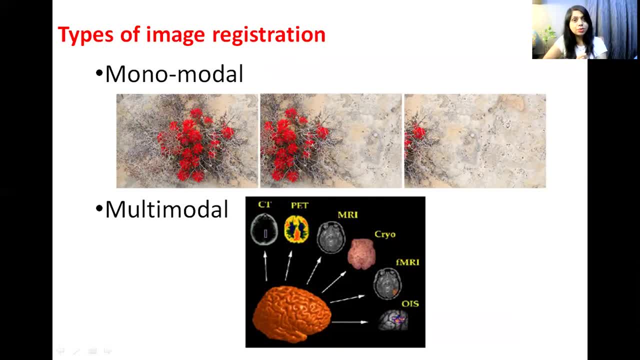 registration when we establish a correspondence between the two images which are captured by two different sensors. that means one is city image and another respect image, or one is paid, another is mri, or one is city and another is mri. that means if these images are captured by different type of 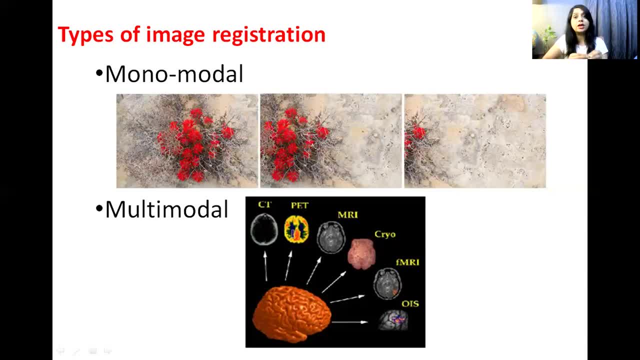 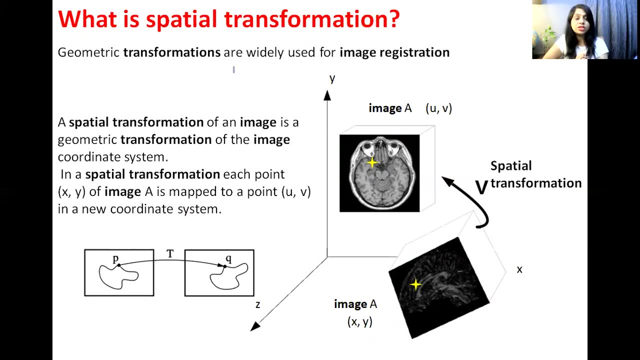 sensors, different type of cameras, and when we try to bring the correspondence, when we try to bring these two images into same coordinate system, then it is said that it is multi-model image registration. now, what is spatial transformation? just now, we have used the word special transformation in the 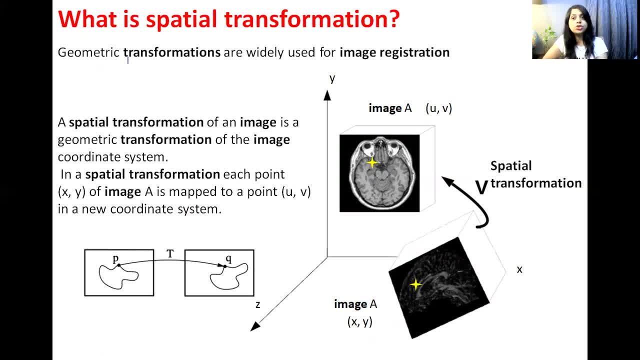 previous slide. what is special transformation? geometric transformations are widely used for image registration. that means these transformations, spatial transformation or geometric transformations. it is used for image registration. So what is spatial transformation? A spatial transformation of an image is a geometric transformation of image coordinate system. Geometric transformation of image coordinate system. 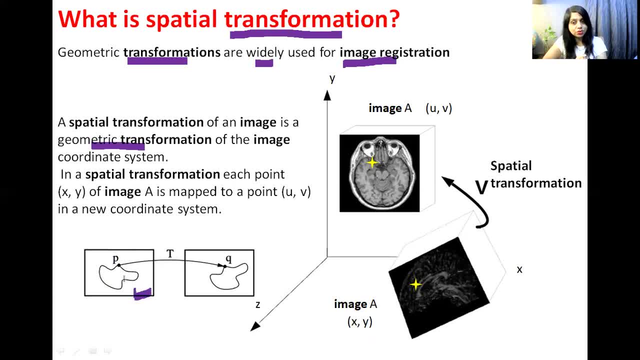 The way I have explained you in this example. this is one image in which the object is same. This is another image. object is same, but object is displaced in X and Y direction. The object is rotated also and it is slightly. it has slightly changed its shape as well, But still P point is available, or pixel P is available in this image. Same pixel P is also available in this image. 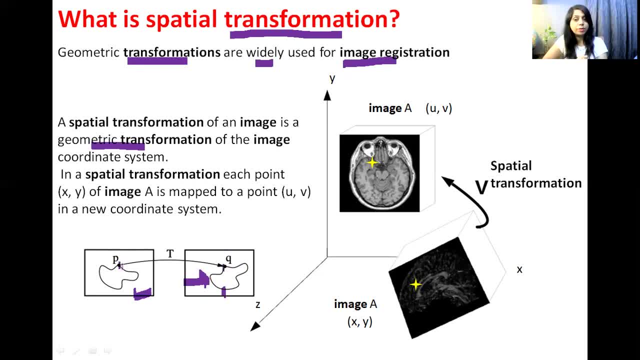 So this is spatial transformation, Spatial transformation of pixel P into pixel Q. That means here the coordinates of pixel P are different and here the coordinates of pixel Q are different, and this is known as spatial transformation. In spatial transformation, each point XY, each- this is image A- each point XY of image A is mapped to a point UV in this. Here the coordinates will be Q, U, V into new coordinate system. 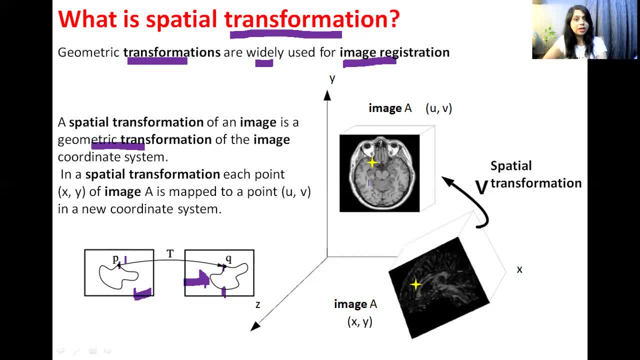 Now, here you can see an example. This is an image of brain: Same thing. This is some another view. The camera is different, The sensor is different, The view angle is different. You can see here: this is X axis, Y axis and Z axis. Entire thing is different. And this is image of same brain, but it is captured from some different view angle, from different depth. maybe That means different distance from the point. Now, here you can see an example. This is an image of brain: Same thing. This is some another view. The camera is different, The sensor is different, The view angle is different. You can see here: this is X axis, Y axis and Z axis. Entire thing is different. And this is image of same brain, but it is captured from some different view angle, from different depth maybe. 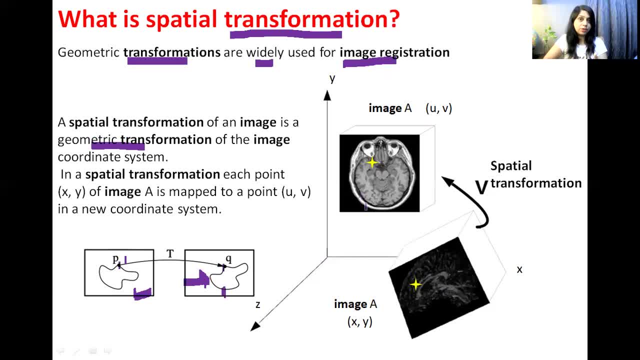 That means different distance from the object or from different angles, Or it is displaced in X direction or Y direction. So images of the same brain, but you can see the images are completely different because angle of view is different, And this is known as spatial transformation. 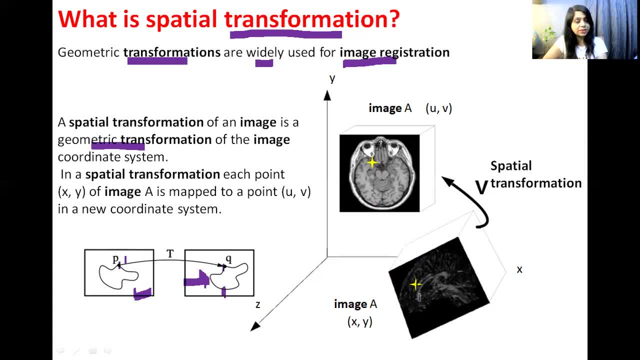 Here, image A: if you say the coordinate of this particular pixel is X, Y, then in this image the same point will lie. Then in this image the same point will lie somewhere here and here the we will say that its coordinates are u, comma, v. this is known as spatial. 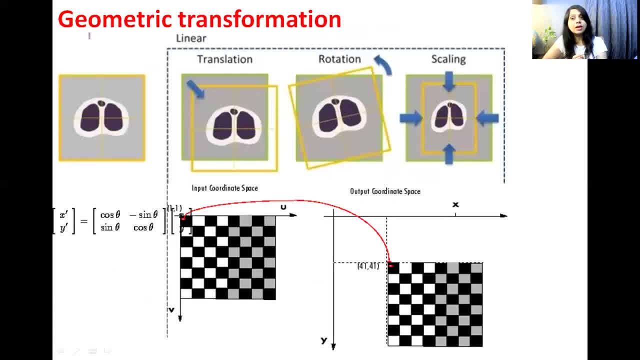 transformation. now, what is geometric transformation or what is spatial transformation? same thing, geometric or spatial transformation. suppose this is image of some object. now there are two types of transformations, that is, linear and non-linear. let's see what are the linear types of transformation. the first one is translation. what is translation means here? you can see that this is image, you know. 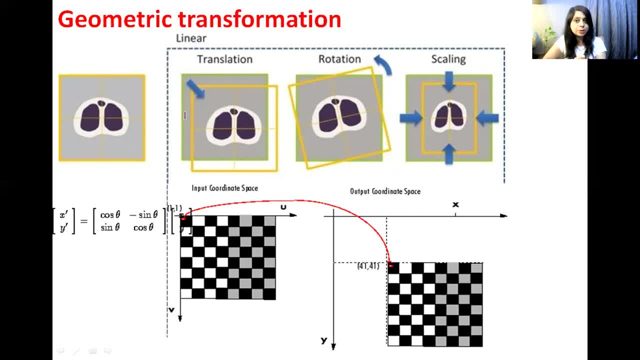 here. this is same image, but now camera is displaced in x direction as well as it is displaced in y direction. that means you can see that in the first image this is original image. in this original image, suppose picture is captured from this point. then what happened in translation? 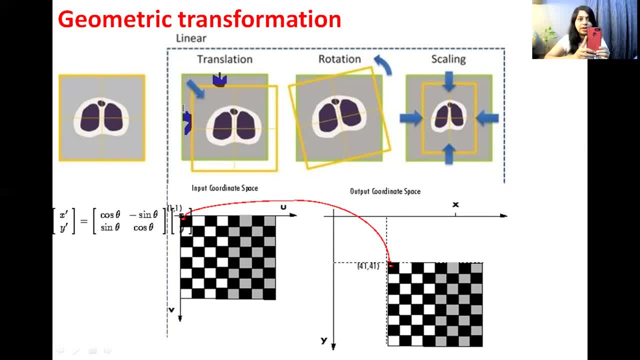 the camera is displaced in X direction, like this, and it is also translated in Y direction, like this, and then captured the image of same object. So here the coverage of image will be completely different. It will not be exactly like this, but it will be like this. Here it is shown with the example. 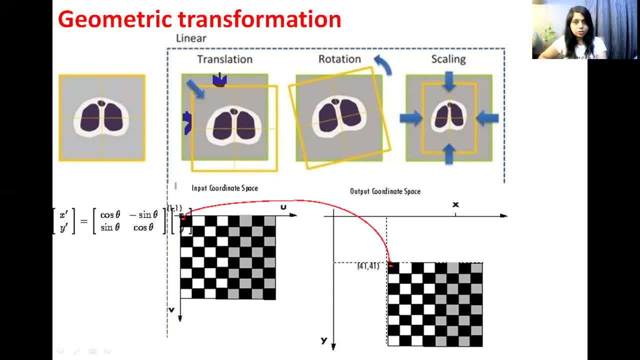 you can see here. This is a check board image. You can see here this is given point a, pixel p. it's coordinates are one comma one, and now it is displaced in X direction like this. It is displaced in Y direction like this, and here the coordinates of same points are 41. 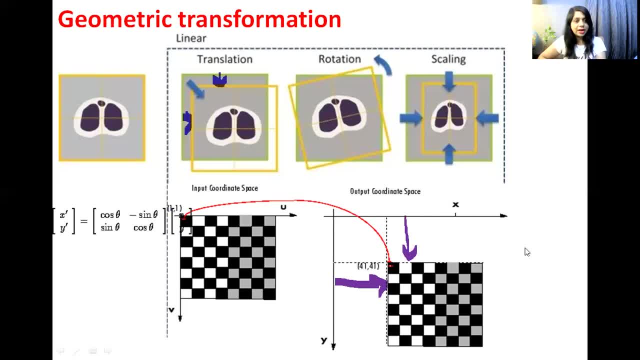 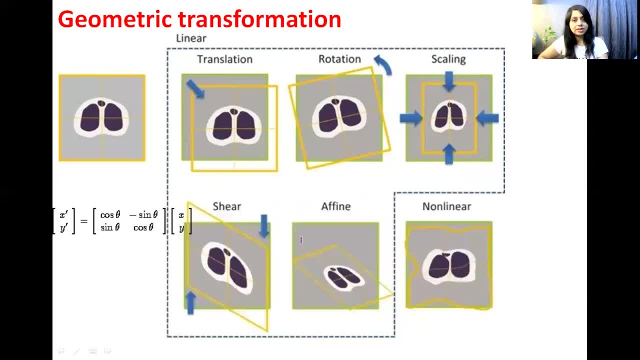 comma 41. So you can say that this is known as translation. This particular geometric transformation is known as translation. The second: you can see that this is rotation Here. when image in this, when image is captured in this particular geometry, it is called rotation. So this is called rotation. So. 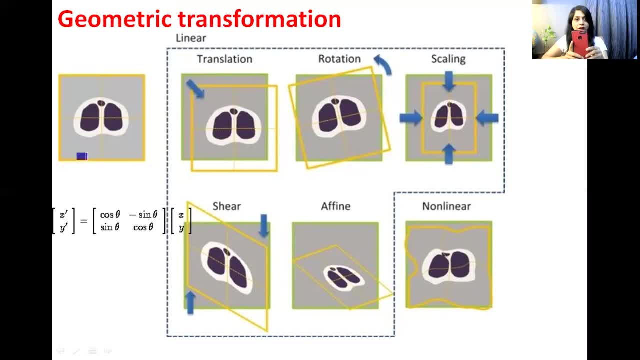 in this angle. in rotation, the camera. camera is slightly rotated like this and then captured the image, So coverage will be obviously different. This is known as rotation. What is scaling? Scaling means when the image is captured from different distance. One is you can say a close. 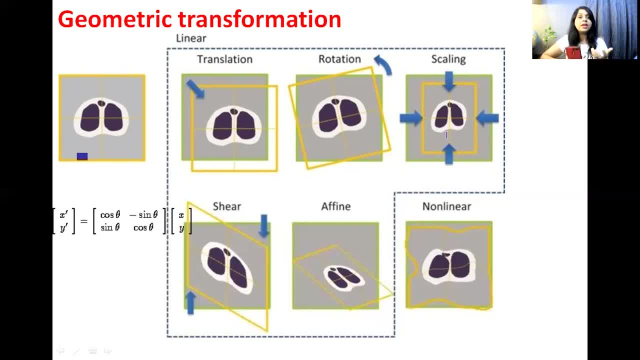 view or a far view, Then scaling will happen. Here you can see that the object is smaller image because there is a scaling. Now, here you can see that this is sheer. Sheer means what happens. the camera is tilted like this. It is. it is like this and then captured the. 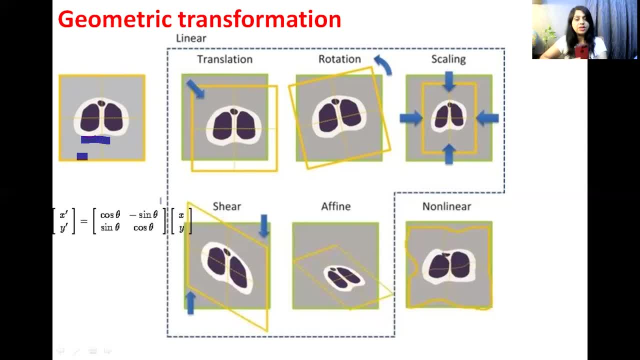 image of same angle, So this is known as sheer. So image will appear as if it is stretched. Then this is a fine transformation. What is the meaning of a fine transformation? Here you can see that the image is translated, rotated and stretched. This is known as a stretch. 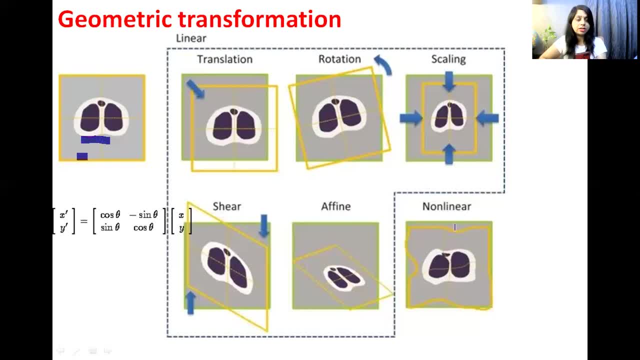 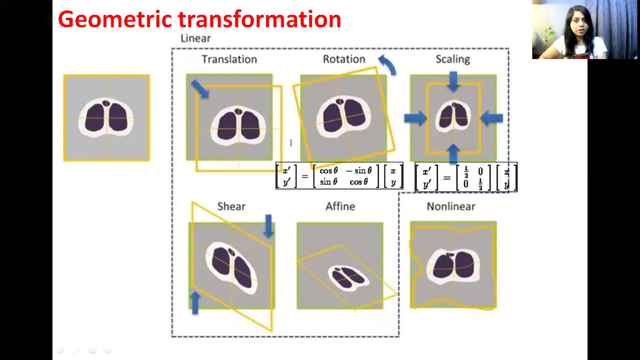 This is known as a fine transformation, and nonlinear transformation means it is a very bad kind of transformation. This is one formula which is used to correct the rotation. that I will explain in the next slide. Now, what is geometry transformation? Let's take an example of this image. It is rotated. Suppose this image is rotated by angle theta. So what? 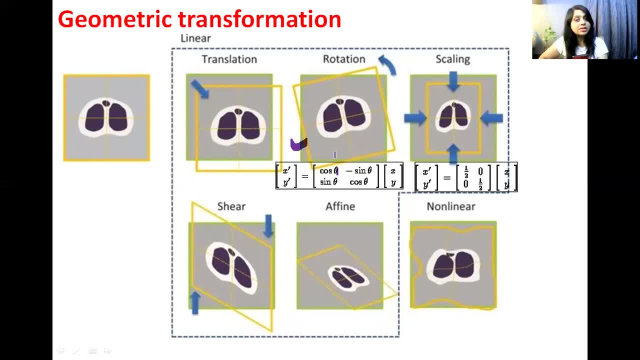 we have to do? first we have to calculate this theta angle- What is value of theta? And then, if we use this formula, we can correct this image into this image. That means, if we apply this formula onto this image, we will get this original image. lattice required. 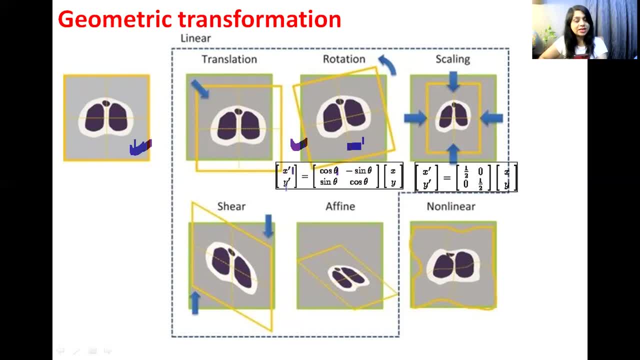 image or base image. What is x, dash, y, dash, x, dash, y, dash, r? These are the pixels coordinates, pixel coordinates of output image. This is cos theta. It is angle by which the camera is rotated, And this is x and y are the pixels of this. 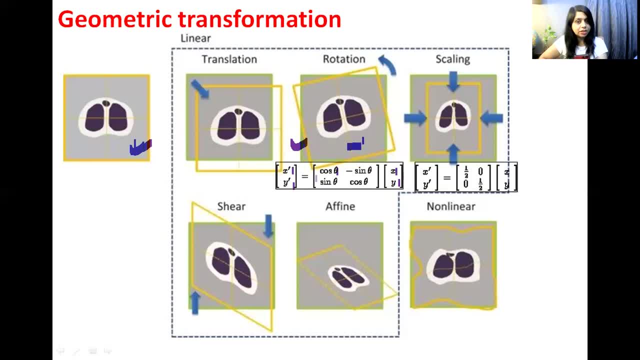 So what we will get when we apply this formula on this image, we will get this image. So this is x, dash, y, dash, r coordinates of output image. This will be our input image. Similarly for scaling, here it is given: if it is scaled, image is smaller or image is bigger, And if 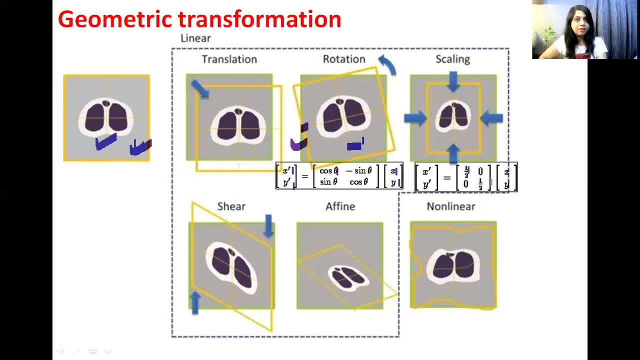 you want to make it small, then here half is given. If two images, one image is double than the other image. That means, if there is, Okay, Exact scaling of doubling, then we can use this formula to bring one image into another. 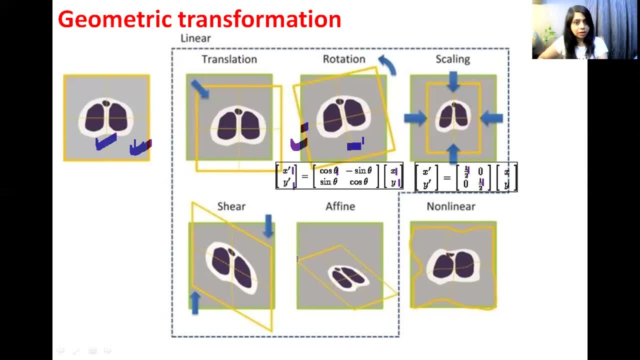 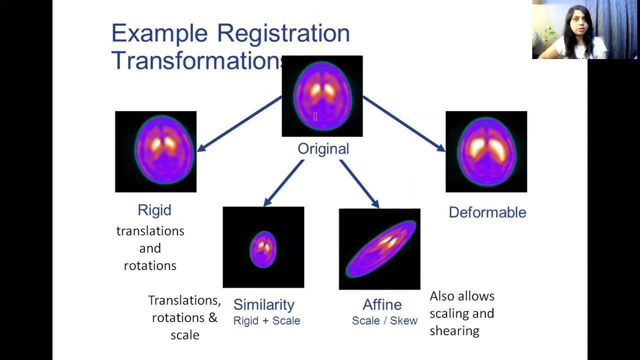 image size. Others I have already explained. I have not included the formulas here because I will take a separate video for geometric transformation. Now, example of registration transformation. You can see that this is some image which is the original image captured by one particular angle by a camera. Now what is this? This? 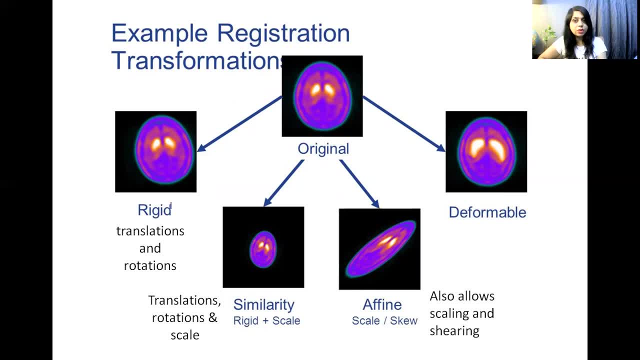 is actually a rigid-body transformation. What is the rigid foreign? That means when the film upstairs in terms of there is translations. translation means displacement in x direction and y direction and rotation. rotation means object is rotated, camera is rotated, then it is said that it is a. 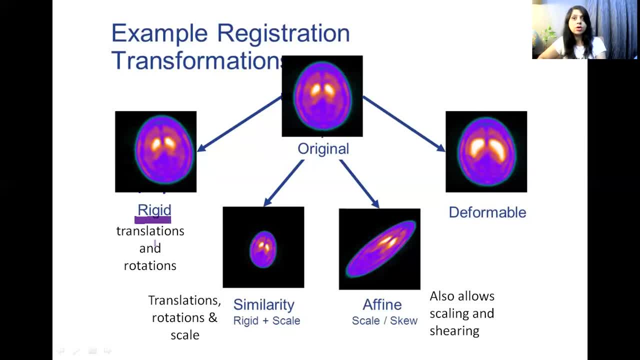 rigid body transformation. what is rigid body transformation? a combination of translation and rotation. now, if you observe this image, what happened? it is translated in x direction. it is rotated. it is translated in y direction. it is rotated, it is rotated in another direction. now, here it is. rotation is in this direction. in this image, the rotation of object is in this direction. 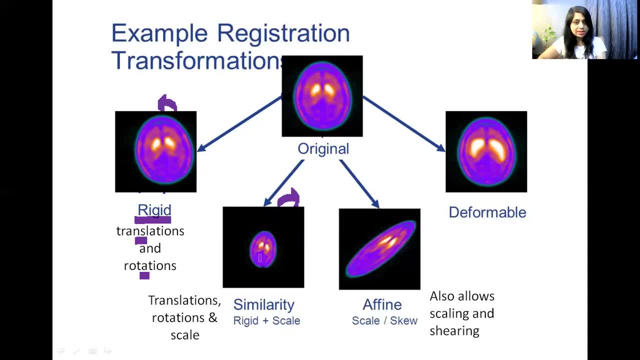 you can see here, here rotation is in this direction and there is a scaling also. that means if there is a combination of translation, rotation and scaling, then it is said that it is a similarity. transform, these are the names of transformations, these are name of spatial transformations. so these, if there is a combination of translation, rotation and scaling, then it is said that it is. 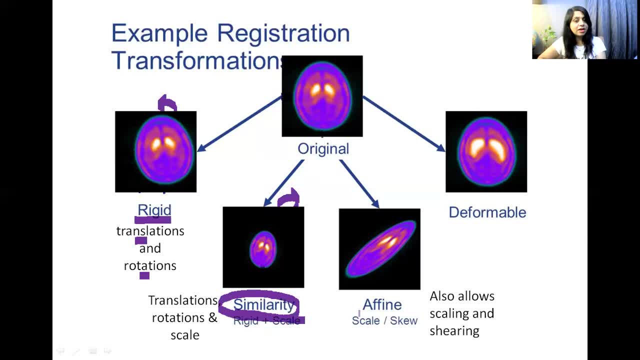 similarity transformation and next is affine transformation. what is affine transformation? you can say that it also allows scaling and shearing. that means there is a translation, there is rotation, there is scaling and there is shearing. when all type of transformations are there, then it is said that it is affine transformation, and it is very difficult. 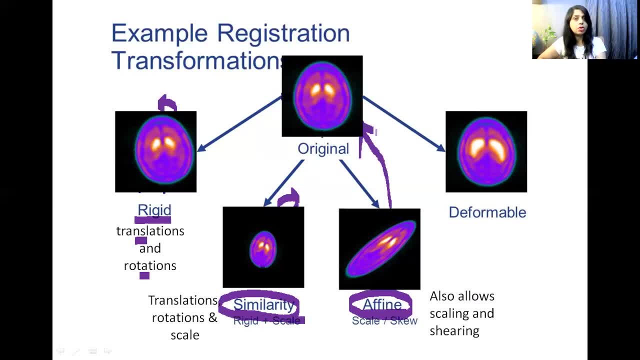 to correct this image and bring it to normal. but it is possible with some formulas we have to use, and here you can see there is a deformation, the object is deformed. there is no rotation or there is no scaling or no, nothing else but only deformation. so these are the types of transformation. 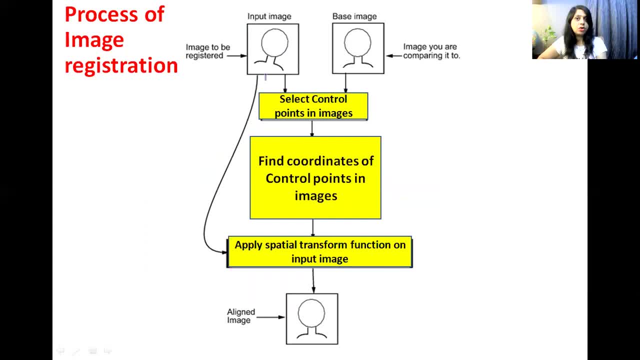 now, what is the process of image registration? if we want to correct image, you can say this is a input image and this is the base image. we want to correct this image like this. we want to make it correct straight. so first we have to do what we have to do. we have to select control, point there. 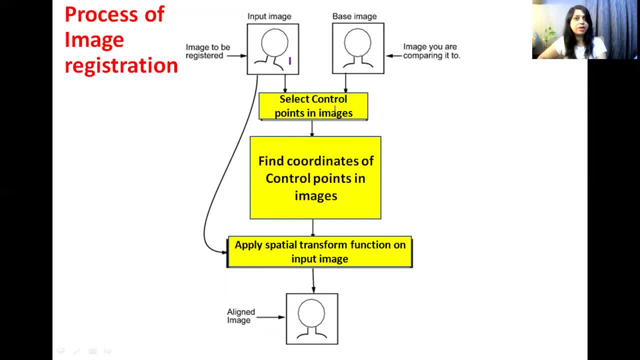 are various methods of image registration. number of methods are available. i am explaining only one type, a simplest type of image registration here. first we have to select control points of the images. that means whatever is: choose some random points in this image and then identify same points in the, this rotary change. then we have input simultaneously: the one which is centriciera, which is 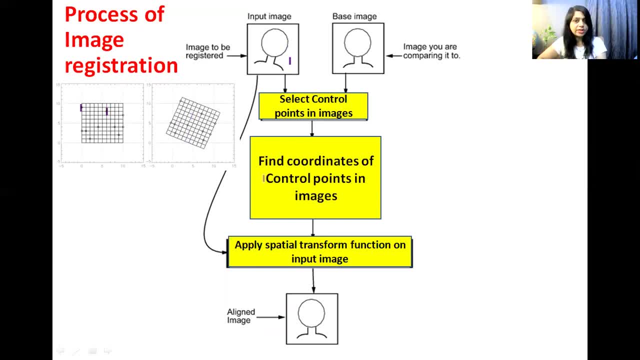 rotated image. these are known as control points. then you have to find out the coordinates of control points in the images. that means find out coordinate of this point. the same point lies here in the second image. find out coordinate of this and this and then use formula to correct. 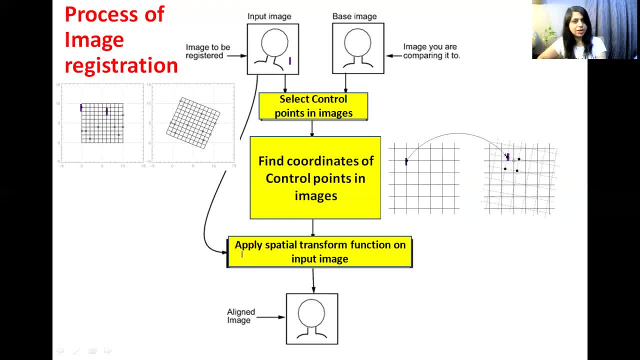 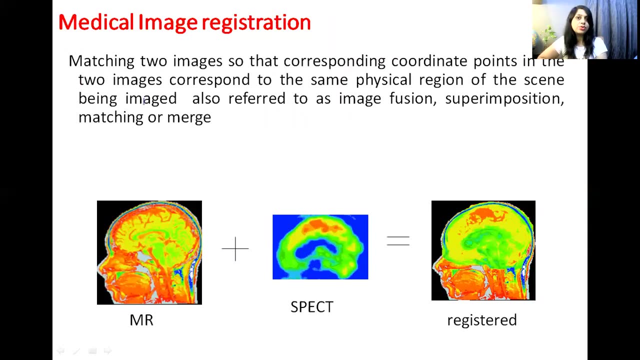 it and then you can transform this image. into this image it is written: apply special transform function- transformation function on input image and you will get this registered image. so this is image registration, which is known as image alignment. now, where it is used, what is the application of image registration? so here i have given an example or application. 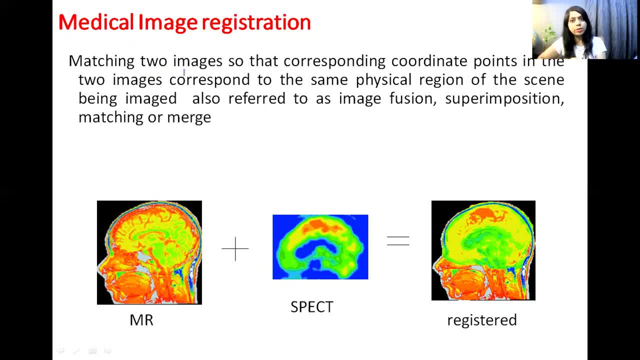 of medical image registration, matching two images so that corresponding coordinate points in the two images corresponds to the same physical region of the scene being image. that means what it means. you can take an example of this image. this is a mri image, mri image of a brain, of a human body, and you can see that here, clearly the boundaries. 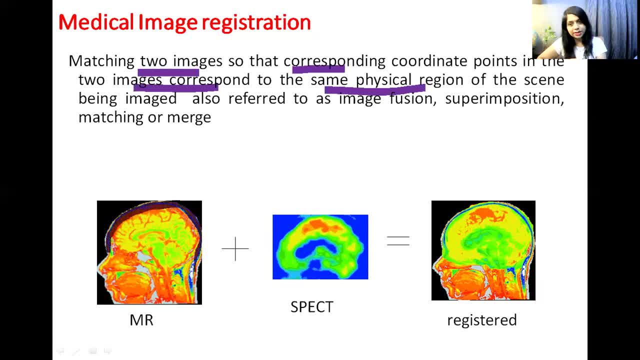 are available. we know where the brain exists. the brain exists here, so this is a brain area. now, this is a spec image. that means it is captured. the brain is same, the human, the subject is same, but it is captured by some different sensor, so it is single photon emission computation. 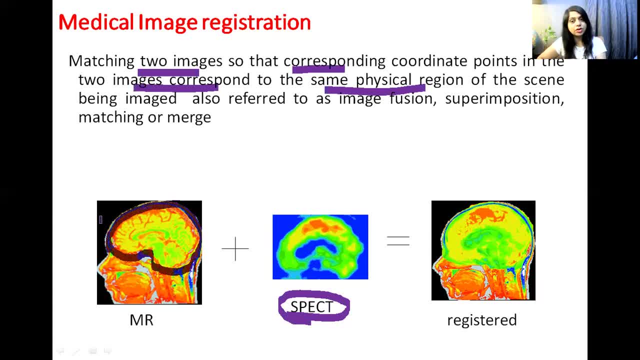 computed tomography. so this is a spec image of the same object which is the same object, but you can see there the boundaries of the brain are not clear. we don't know, but here tumor is clearly visible. in this image tumor is not clearly visible. you can see again in: 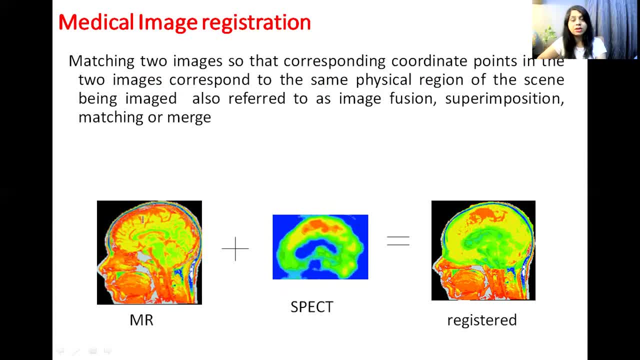 this image, this tumor is clearly visible and here tumor is not clearly visible. so this image is not giving a complete information. this image is also not giving complete information because here tumor is clearly visible. we don't know the location of image. so, in that case, what we, what we can do, 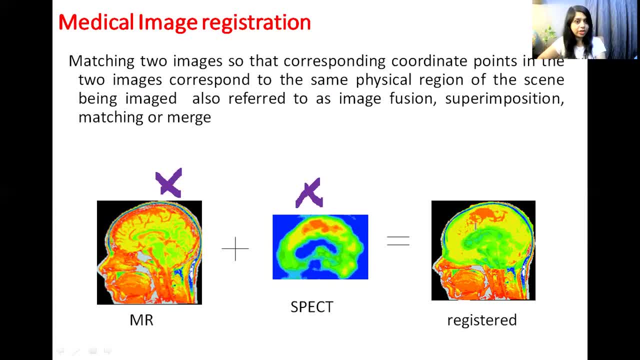 add these two images. we can fuse these two images so that we can clearly see the tumor. we can also identify where exactly this tumor is available from the boundaries of brain, because in this the boundaries are clear and here boundaries are not clear. but for fuse, fusing of these two images, we 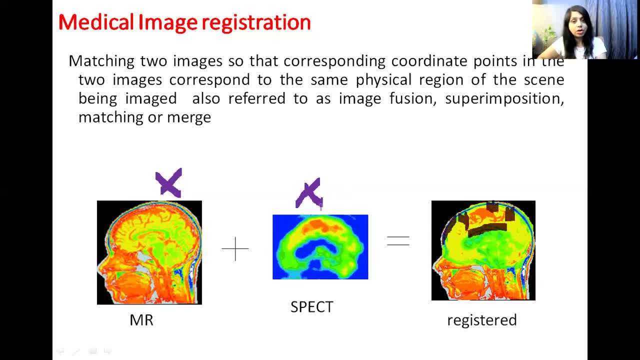 need to register them. we have to properly align them. we cannot align them like, like this. if we align it like this and then if we can see the tumor here, it is of no use. so for fusion, we need to register the images. we have to exactly find out, suppose this point. so where this point is available. 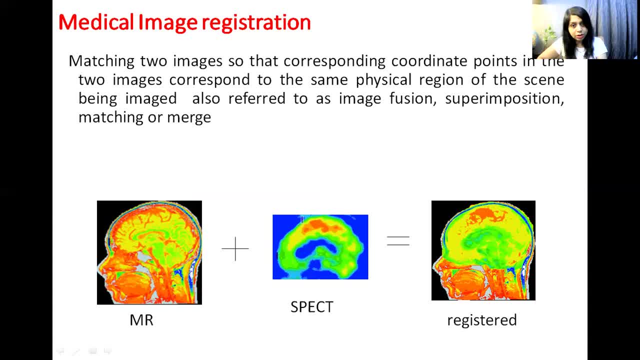 in this image. so we have to find out coordinate of this particular point. so if i identify where this particular point is available in this image, or this particular point where this particular point is available in this image, and then we have to align, we have to bring both the images. 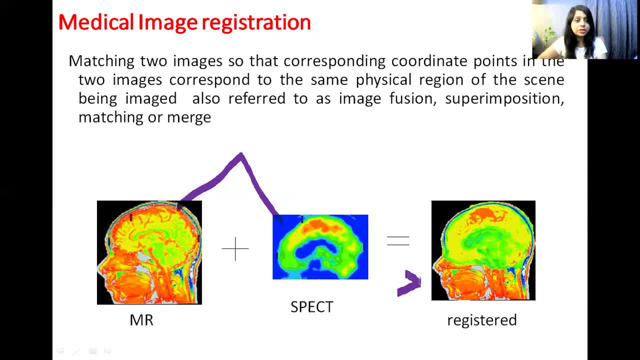 in the same coordinate system and then only you can add these two images. so bringing these two different type of images in the same coordinate system is known as image registration, and fusing is is an application. fusing of image is an image registration application. this is another example. 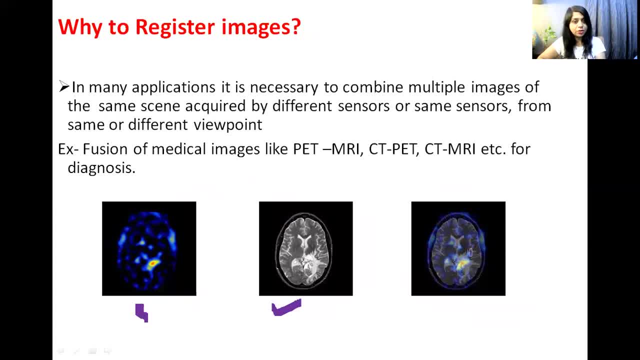 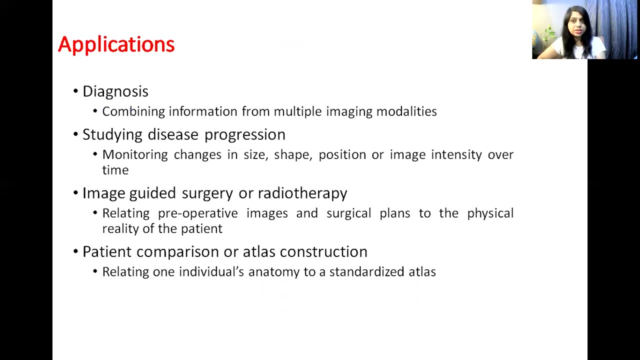 this is also spec image and this is mri image and these are fused. you can see here, here the tumor is. when we fuse it is, it gives the exact picture of tumor as well as the anatomy of brain. now, what are the applications of image fusion in medical uh applications? the diagnosis it is used. 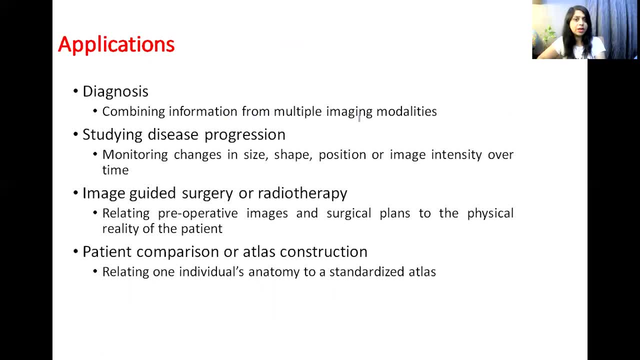 for com, because combining information from multiple imaging modalities gives additional information. when we combine spect and mri or ct and mri or pet image and mri image, then it gives additional information studying disease progression. this is progression means when images are taken at different times. 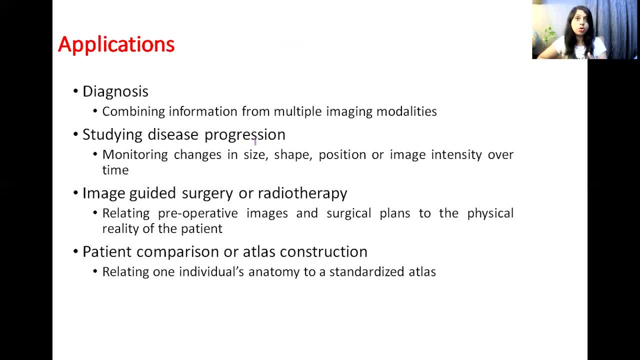 then if there is a deformation or if tumor is grown or it is reduced. that can be analyzed by size, shape and position or image intensity over time. image guided surgery or radiotherapy, where it is used, related to pre-operative images and surgical plans so doctors can plan the 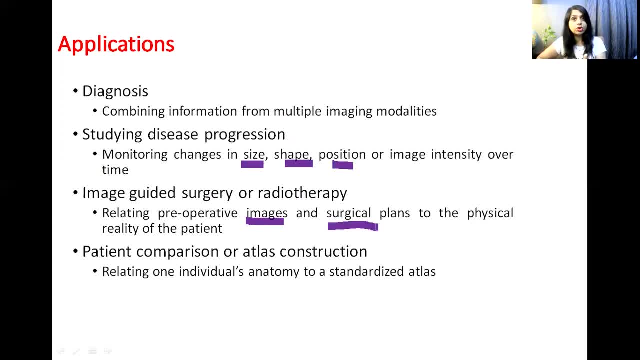 surgeries based on exact location of tumor, where it exists, what is the size of it. so based on that, they can plan their surgery. patient comparison to atlas construction: that means relating one's individual anatomy to a standardized atlas. that means: suppose there is a specific, uh, suppose this. 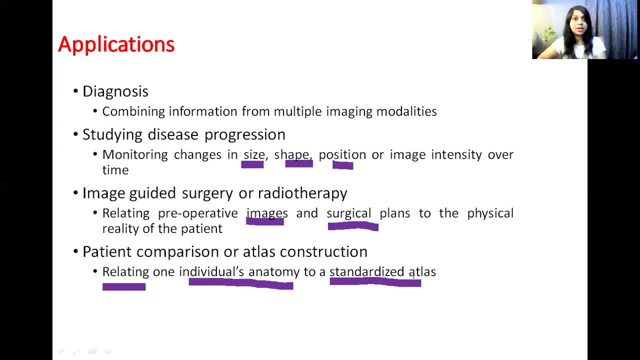 should be a size of brain. so in another person, if size of brain is little smaller, or if it is, uh, bigger than the standard size, then that analysis can be done with this image fusion or image registration. that means comparison of standard one with the individual's anatomy. 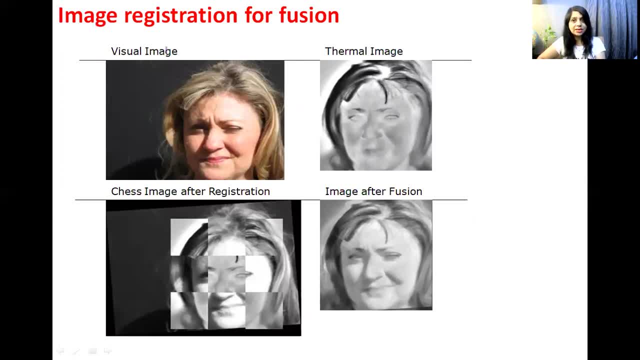 image registration for fusion. this is another example. you can see this is a visual image taken by vr camera, very normal camera. the image is like this and this image is captured by thermal image. generally these cameras are used wherever there is a dark. there is no light for recording, so they 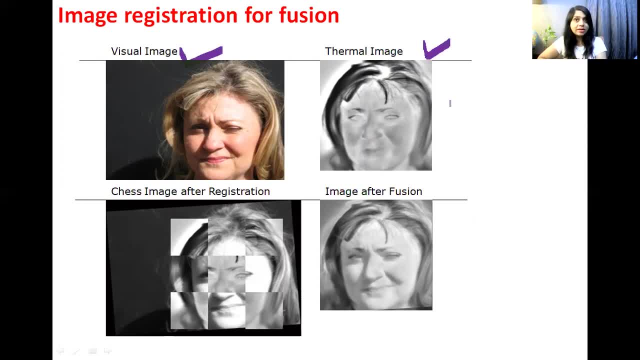 have been used as long as they can record imaging image, that the image shows it clearly. everything can only be captured only by the images taken by the camera. so you have to man light. so thermal image will be like this, so colder part will be seen black and whatever is hot that. 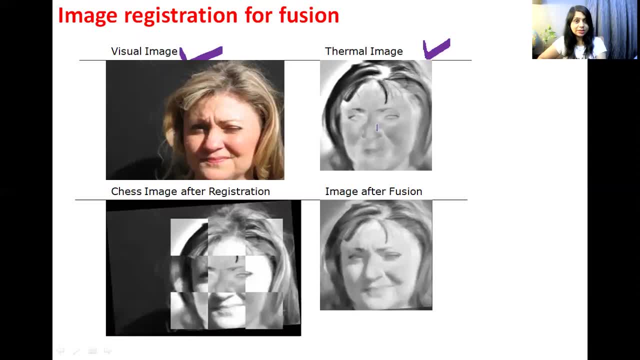 will be seen white, so thermal images can be captured in the dark also. so you can see this kind of image. but here the features are not clear. but when we fuse it we can really identify if it is the same person or not. generally these are used in army or any defense applications. 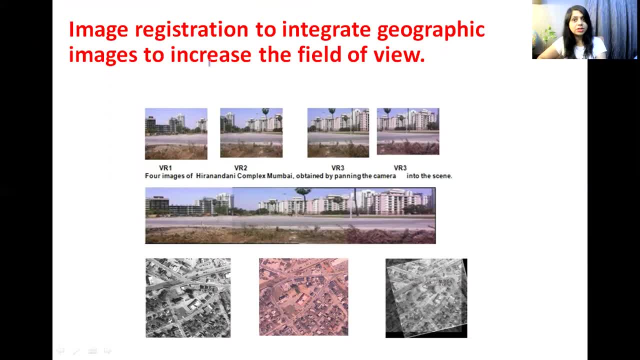 image registration to integrate geographic images, to increase the field of view. view, you can see that these images are taken. this is a hira nandani complex and here of mumbai, and here the camera is spanned from left to right. here the coverage of image is different. 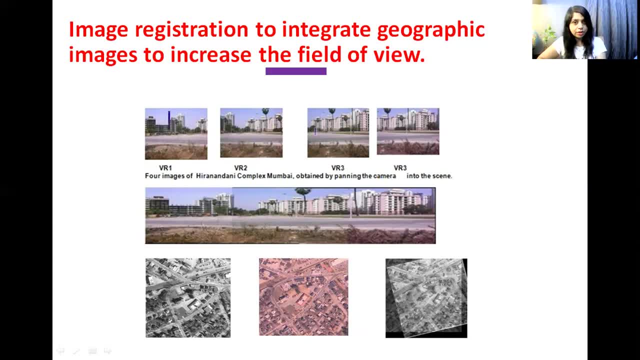 here the image is starting from this point. now, if you see this in this image, it is starting from somewhere like this point and this somewhere it is starting. this is starting somewhere here, and suppose we want to make a mosaic, a panoramic view, out of these different images captured at. 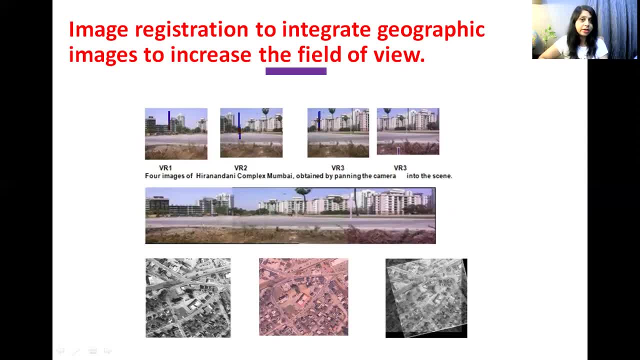 different by panning the camera towards right or in x and y direction, and if we want to generate this view, we have to make a mosaic to identify. what is the coordinate of this in this image? what are the coordinates of these points in this image? what are the coordinates of this in this image? what are the coordinates of? 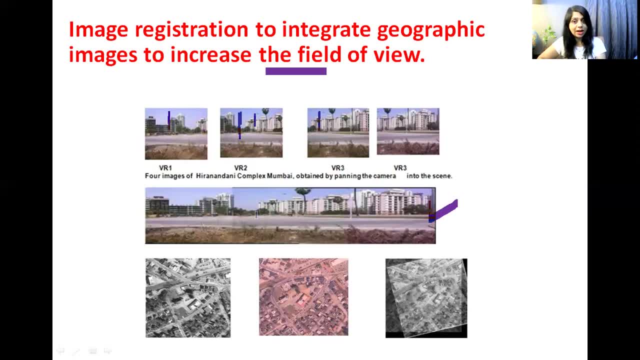 this in this image, and then we can align all these images and we can stitch these images together to get this view. now you will see that if this panoramic mode is already available in the cameras, why to do this image registration and so many calculations for this panoramic view or for